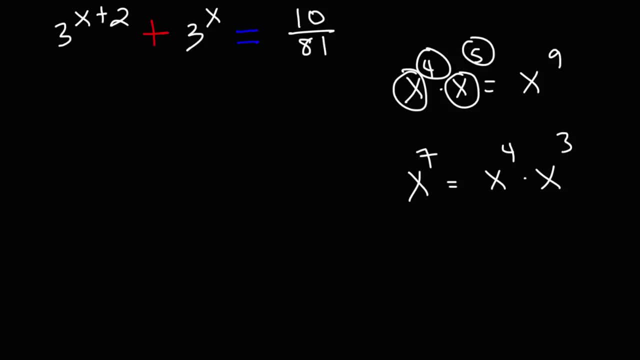 seven. you can break that into x to the fourth times x to the third. Now, what about 3 raised to the x plus 2?? We can add the exponents. We can add the exponents. We can add the exponents. 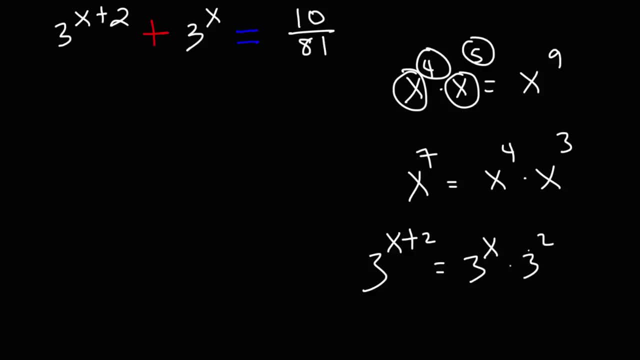 We can write that as 3 raised to the x times 3 squared, because it's x plus 2.. And that's what we're going to do with the first term in this equation. We're going to write it as 3 squared times 3 raised to the x. So now let's get rid of this, And then it's going to be plus 3 to the x. 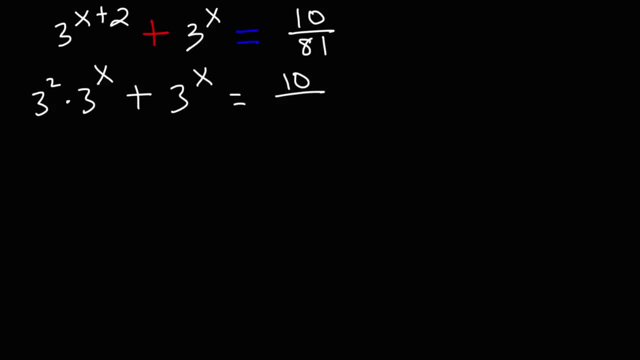 and that's going to equal 10 divided by 81.. Now notice that we have a lot of 3s on the left side. An 81 is a multiple of 3.. So what we want to do is change 81 into something or into a base 3.. 3 to the fourth power is 81. It takes four 3s. 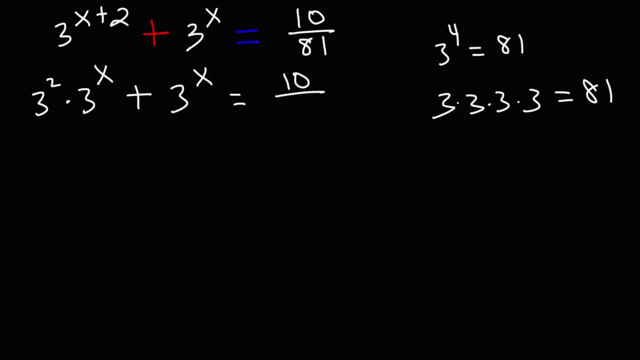 multiplied to each other to get to a value of 81.. So let's replace 81 with 3 to the fourth power. Now, what do you recommend that we should do at this point? What is our next step? Well, for starters, we can do something with 3 squared, 3 squared or 3 times. 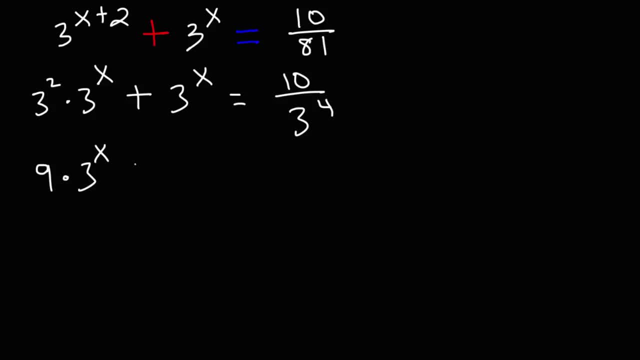 3 is 9.. So we have 9 times 3 to the x plus 3 to the x. Now we can write this as 3 to the x times 1, because it's just 3 to the x, And we'll talk about why we're going to do that in a moment. 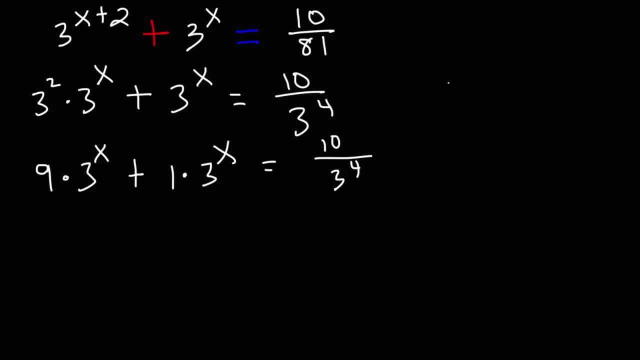 Now let's say, if we have 5x plus 3x, If the base is the same or if the variable is the same, we can add the coefficients. So 5 plus 3 is 8x. Notice that we have the same variable here. 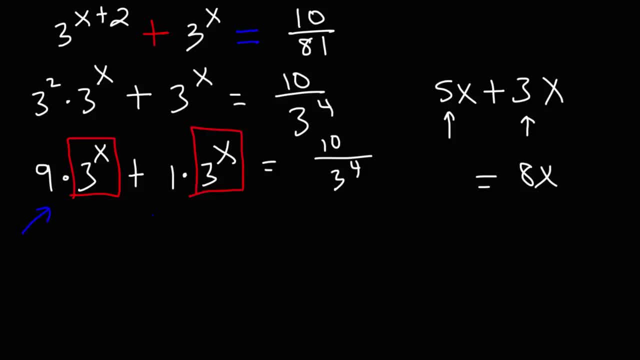 3 to the x. So what we can do is add the coefficients: 9 plus 1 is 10.. So we have 10 times 3 raised to the x, And that's equal to 10 times, or rather divided by 3 to the fourth. But what we're going to do at 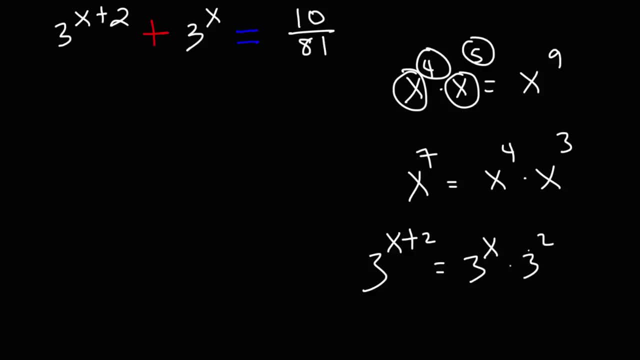 We can write that as 3 raised to the x times 3 squared, because it's x plus 2.. And that's what we're going to do with the first term in this equation. We're going to write it as 3 squared times 3 raised to the x. So now let's get rid of this, And then it's going to be plus 3 to the x. 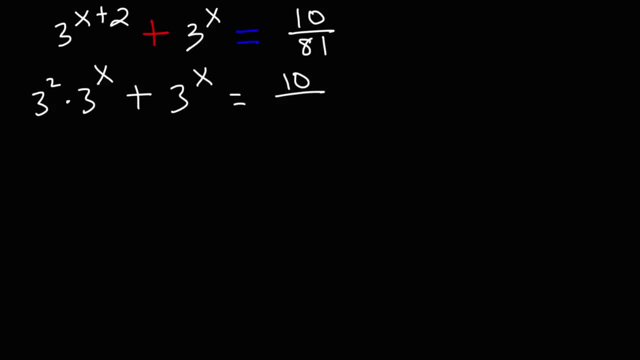 and that's going to equal 10 divided by 81.. Now notice that we have a lot of 3s on the left side. An 81 is a multiple of 3.. So what we want to do is change 81 into something or into a base 3.. 3 to the fourth power is 81. It takes four 3s. 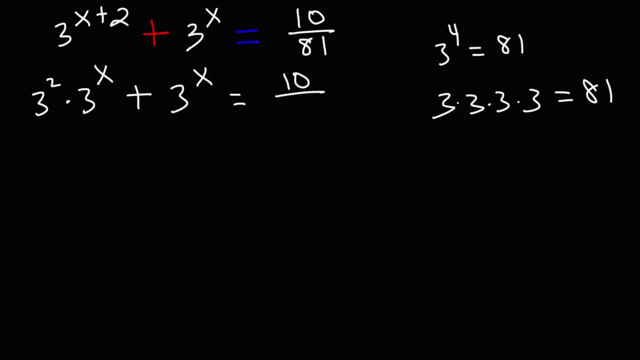 multiplied to each other to get to a value of 81.. So let's replace 81 with 3 to the fourth power. Now, what do you recommend that we should do at this point? What is our next step? Well, for starters, we can do something with 3 squared, 3 squared or 3 times. 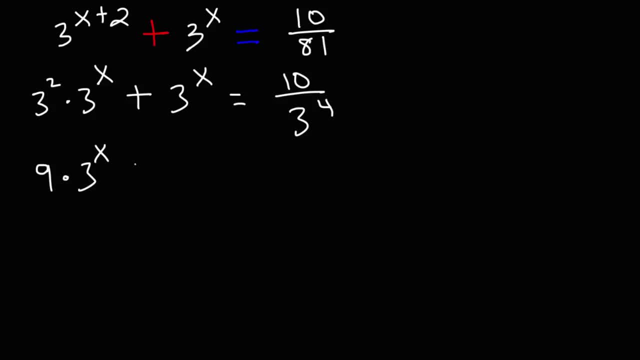 3 is 9.. So we have 9 times 3 to the x plus 3 to the x. Now we can write this as 3 to the x times 1, because it's just 3 to the x, And we'll talk about why we're going to do that in a moment. 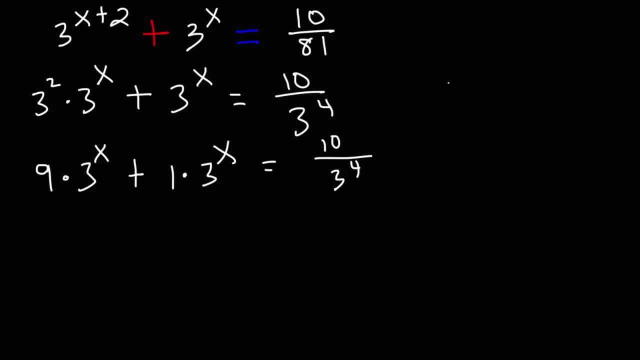 Now let's say, if we have 5x plus 3x, If the base is the same or if the variable is the same, we can add the coefficients. So 5 plus 3 is 8x. Notice that we have the same variable here. 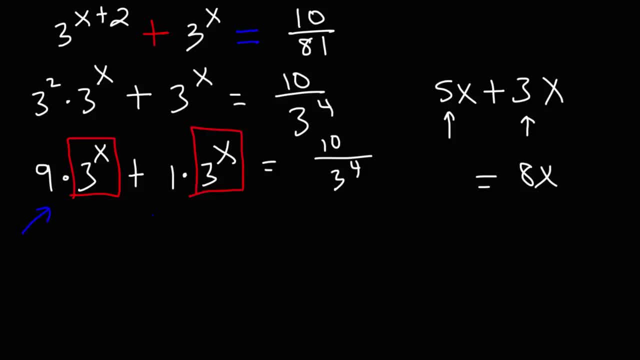 3 to the x. So what we can do is add the coefficients: 9 plus 1 is 10.. So we have 10 times 3 raised to the x, And that's equal to 10 times, or rather divided by 3 to the fourth. But what we're going to do at 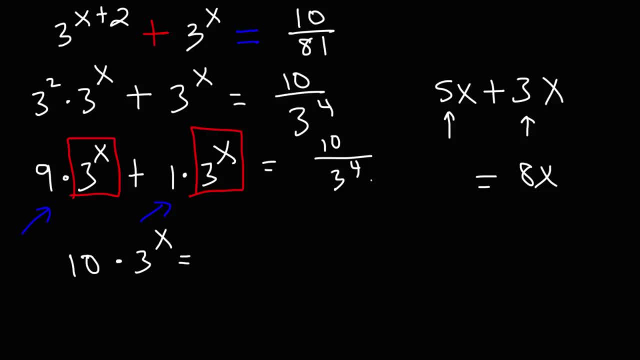 this point is we're going to move the 3 from the bottom to the top of the fraction. If we do that, what's going to happen to the exponent? The exponent is going to change sign. It's going to change from positive 4 to negative 4.. And that's a property of negative exponents, For instance, 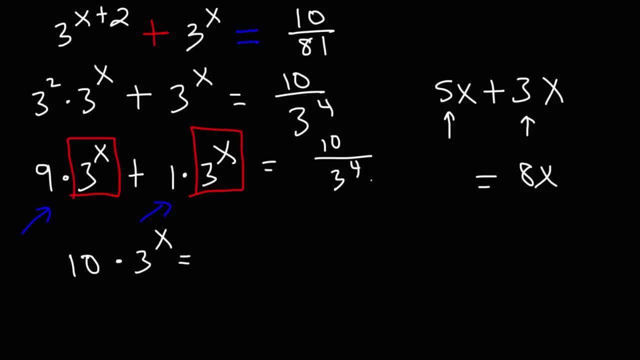 this point is we're going to move the 3 from the bottom to the top of the fraction. If we do that, what's going to happen to the exponent? The exponent is going to change sign. It's going to change from positive 4 to negative 4.. And that's a property of negative exponents, For instance, 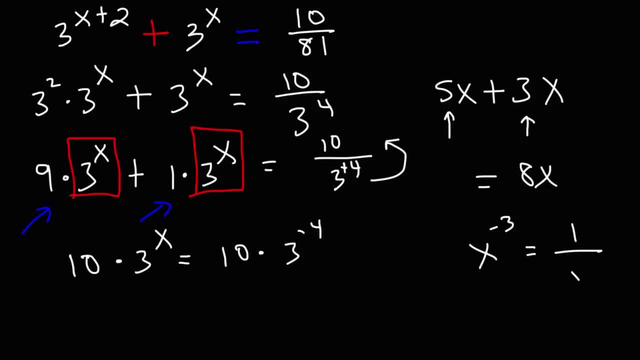 x to the negative, 3 is the same. So we're going to add the coefficients, So we're going to add the same as 1 over x to the positive 3.. So whenever you move a variable or a number from the top to 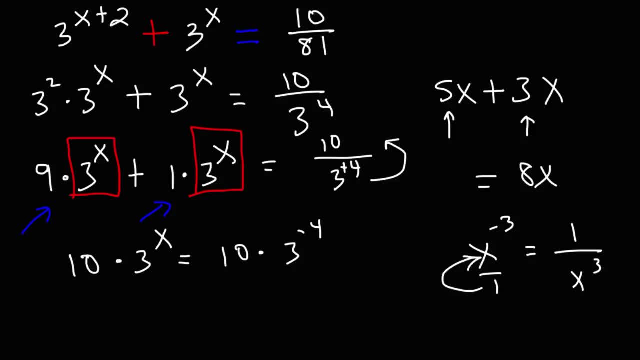 the bottom, or from the bottom of a fraction to the top, the exponent will change sign. So that's one of those algebra rules that you just have to commit to memory. So now we're almost done. We're almost finished with this problem. So what do you think? our next? 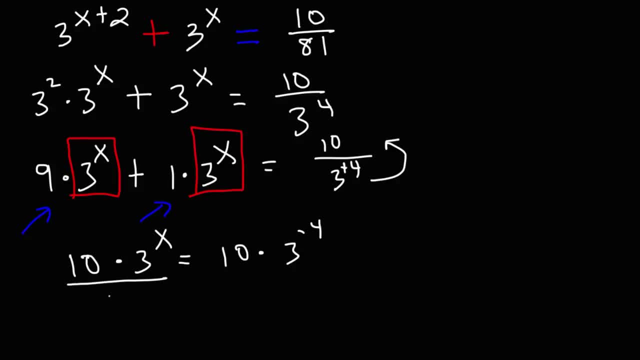 step is here. Our next step is to divide both sides by 10.. Once we do that, we're going to be left with: 3 raised to the x is equal to 3 raised to the negative 4.. Now notice that the bases are the same. We have base 3 on the left side. 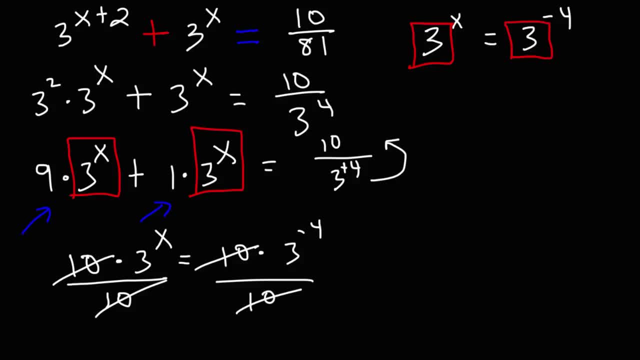 and on the right side of the equation, If the bases are equal to each other, then that means that the exponents are the same. So we're going to divide both sides by 10. And that's going to be must be equal to each other. So therefore, x is equal to negative 4. And this is the answer to. 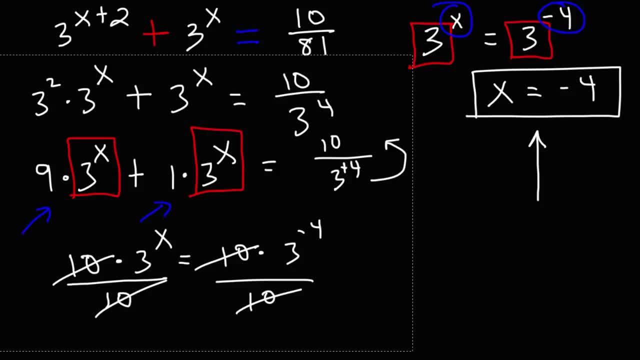 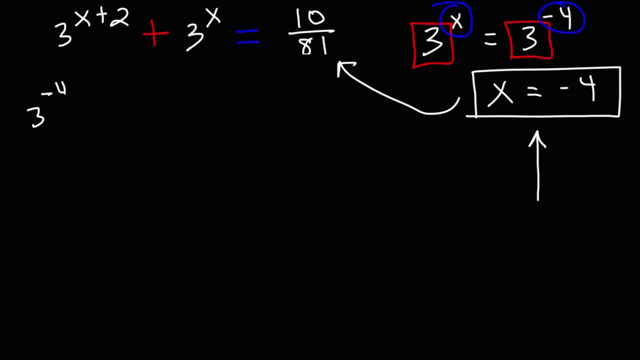 the problem. Now, what we can do is we can make sure that we have the right answer by taking this value and plugging it into the original equation. So let's do that. Let's replace x with negative 4.. So we have 3 raised to the negative 4 plus 2.. Negative 4 plus 2 is negative 2.. 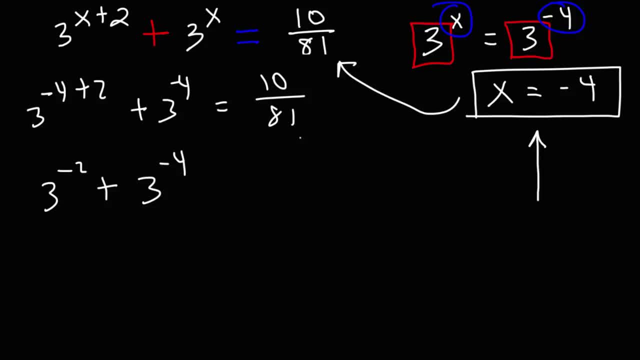 And then we have plus 3 raised to the negative 4.. We're going to see if that equals 10 divided by 81.. 3 to the negative, 2 is 1 over 3 squared. 3 to the negative, 4 is 1 over 3 to the fourth. 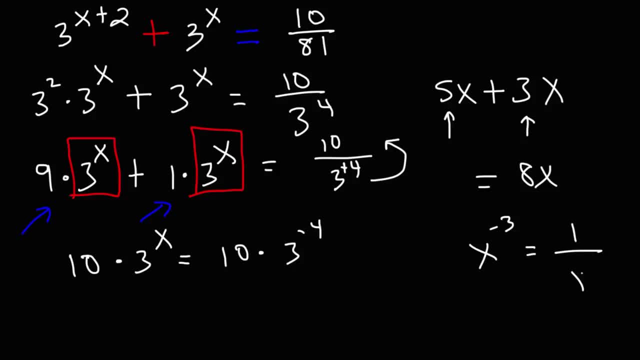 x to the negative 3 is the same as x to the negative 3.. So we're going to add the coefficients, The exponent is the same as 1 over x to the positive 3.. So whenever you move a variable or a number from the top to the bottom, or from the bottom of a fraction to the top, the exponent 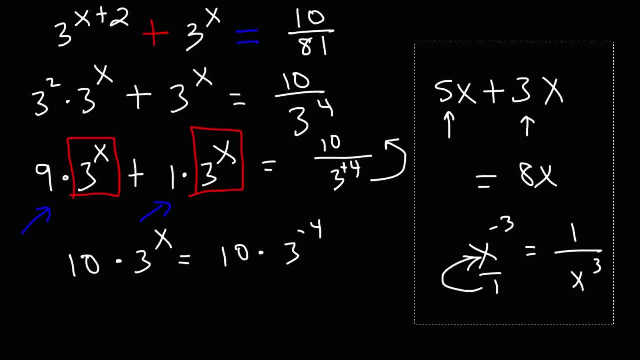 will change sign. So that's one of those algebra rules that you just have to commit to memory. So now we're almost done. We're almost finished with this problem. So what do you think our next step is here? Our next step is to divide both sides by 10.. Once we do that, we're going to be left with 3. 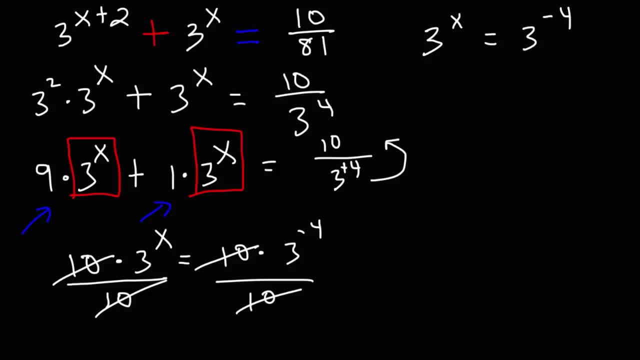 raised to the x is equal to 3 raised to the negative, 4.. Now notice that the bases are the same. We have base 3 on the left side and on the right side of the equation. If the bases are equal to each other, then that means that the exponents are the same, So we're going to divide both sides. 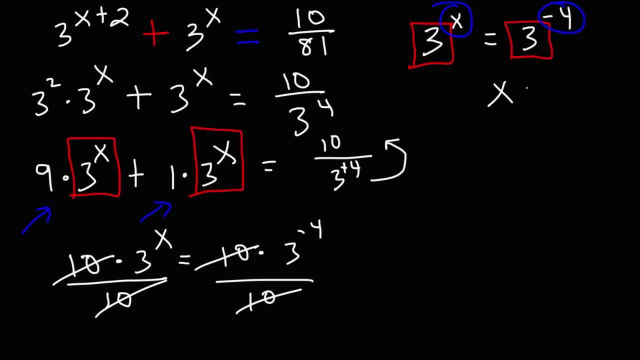 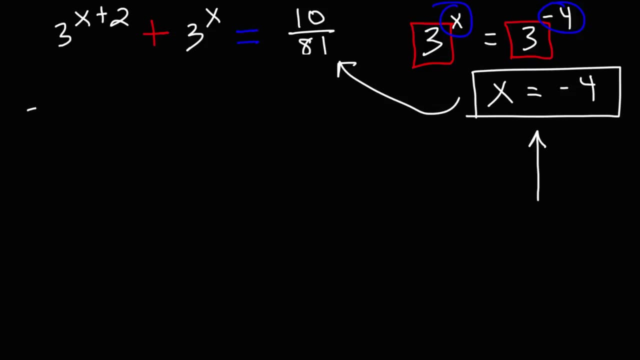 must be equal to each other. So, therefore, x is equal to negative 4.. And this is the answer to the problem. Now, what we can do is we can make sure that we have the right answer by taking this value and plugging it into the original equation. So let's do that. Let's replace x with negative 4.. 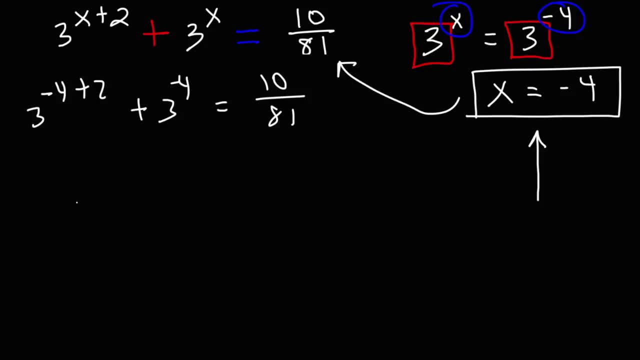 So we have 3 raised to the negative, 4 plus 2.. Negative 4 plus 2 is negative 2.. And then we have plus 3 raised to the negative 4.. We're going to see if that equals 10 divided by. 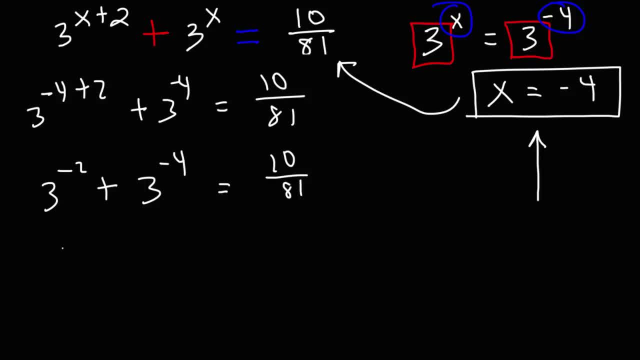 81.. 3 to the negative. 2 is 1 over 3 squared. 3 to the negative, 4 is 1 over. 3 to the 4th, 3 squared is 9.. 3 to the 4th is 81.. And 81 is 9 times 9.. 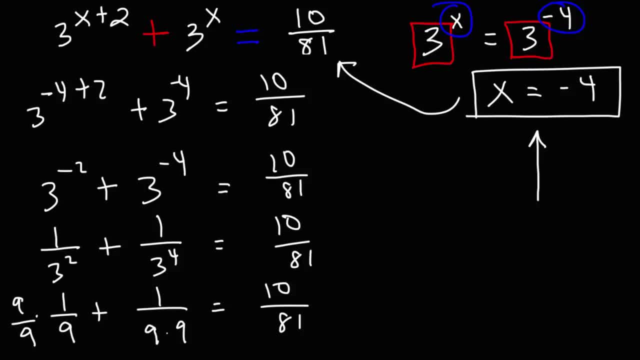 So the first fraction, I'm going to multiply the top and bottom of the equation. So I'm going to multiply the top and bottom of the equation. I'm going to multiply the top and bottom of the equation by 9 over 9.. 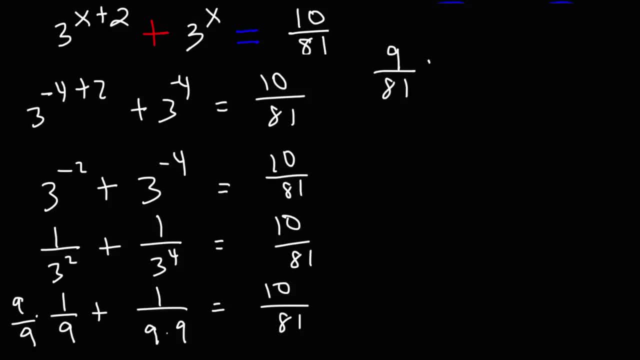 So I'm going to get 9 over 81 plus 1 over 81.. Now, because the denominator of the two fractions are the same, we can now add the numerators: 9 plus 1 is 10.. So the left side is equal to the right side, which means the answer is correct.